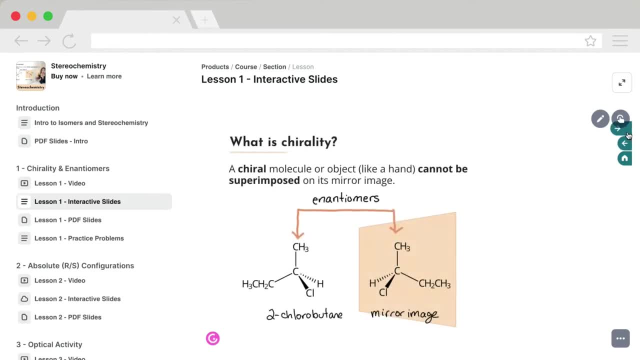 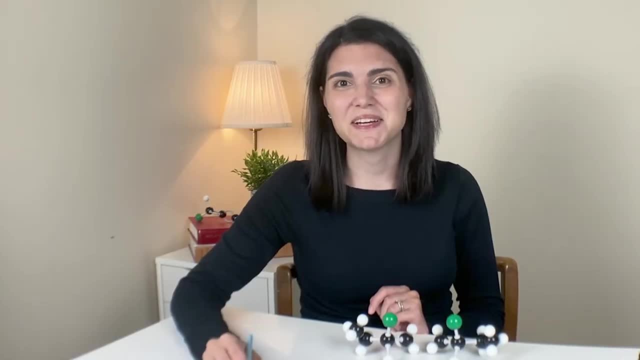 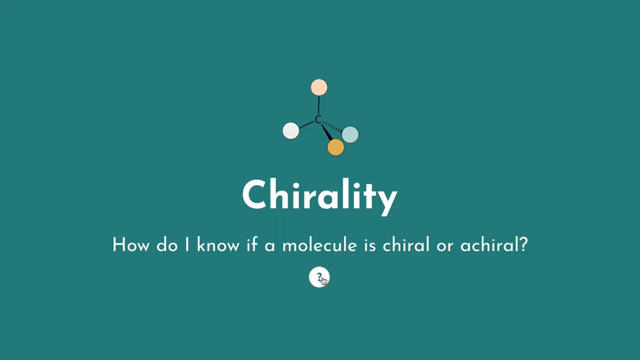 a copy of the slides that I'm using today. just click the link below and, while you're at my website, make sure that you check out all of the other organic chemistry resources that I've got on there. Let's get started. A chiral object is an object that is not identical to its mirror image. 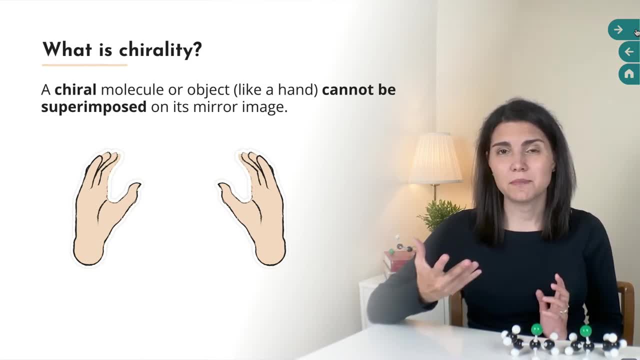 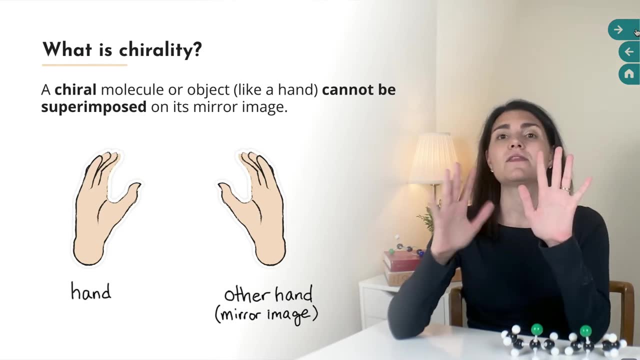 The word chiral comes from the word chiral, which means a particle. A hand is a really good example of an object that is chiral. My hands are mirror images of one another. There's no way that I can superimpose one of my hands perfectly. on the other hand, 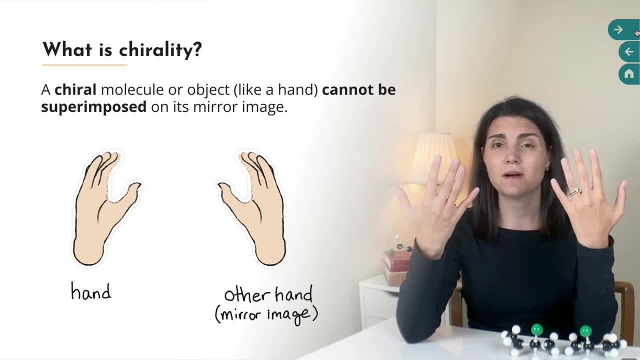 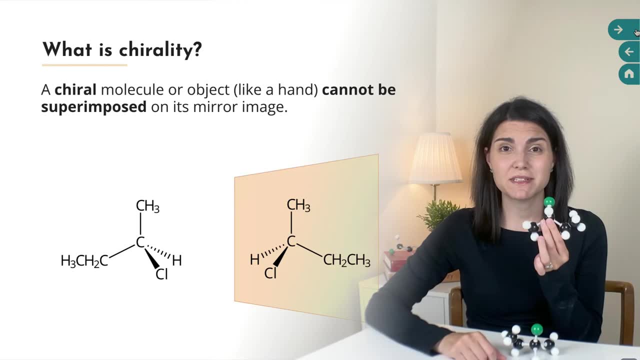 They're not identical, but they are mirror images, and so hands are chiral. Molecules are just very tiny objects and they can be chiral too. For example, this molecule is 2-chlorobutane and it's chiral. This is its mirror image. 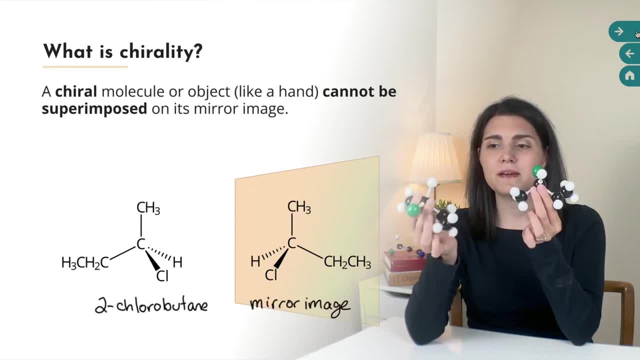 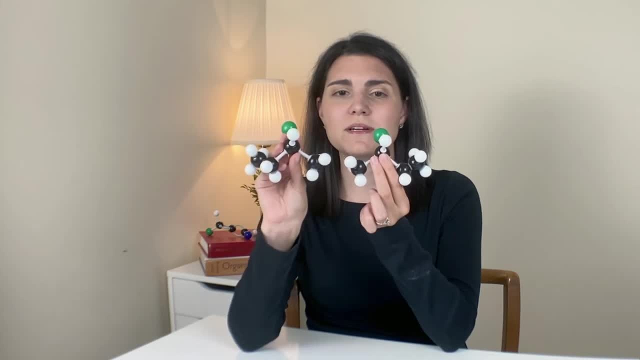 and there's no way that we can rotate or manipulate these mirror images around so that one can be totally superimposed on the other. If you notice, here we've got both hydrogens pointing to the front towards you, both chlorines pointing back, but the alkyl groups are. 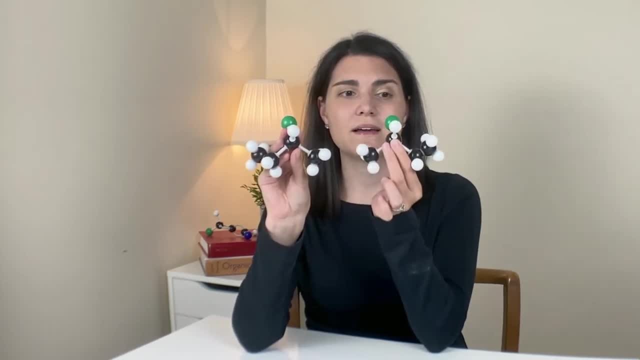 switched. On this side we've got an ethyl over here and a methyl over here, and for this molecule we've got an ethyl pointing this way and a methyl pointing this way. If I rotate this one to put the methyl back in line, we've now switched the direction of the chlorine and the hydrogen. 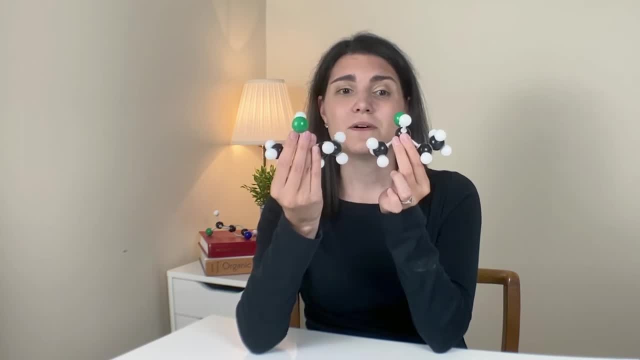 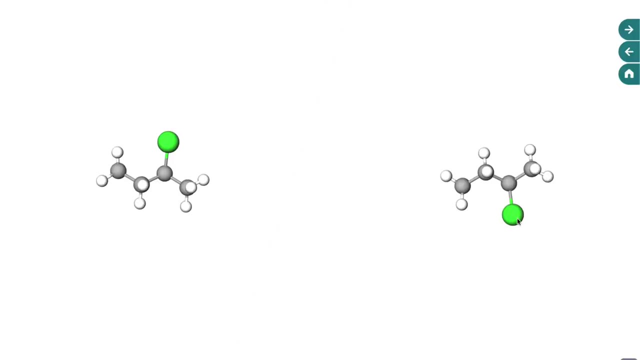 front to back. They're opposite on each molecule, so there's no way we can superimpose these. In case you don't believe me, give it a try yourself. Here are the same two molecules. They are mirror images of each other and no matter how you twist them around. 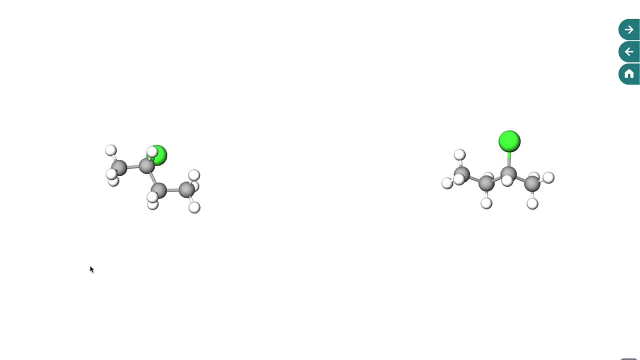 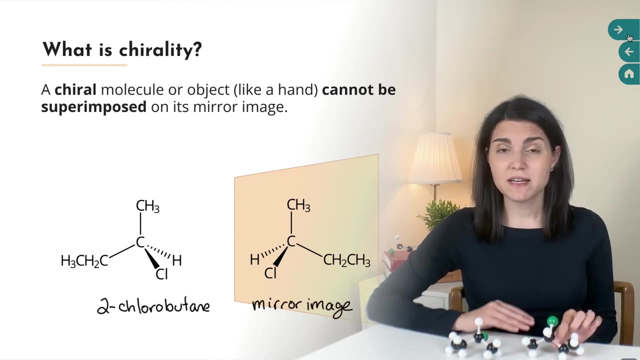 you can't make them line up and look exactly alike, Because 2-chlorobutane can't be superimposed on its mirror image. we say that 2-chlorobutane is chiral, And we use a special word to describe the relationship between these two non-superimposable. 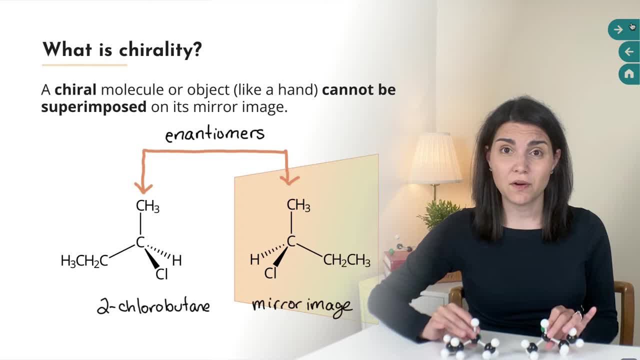 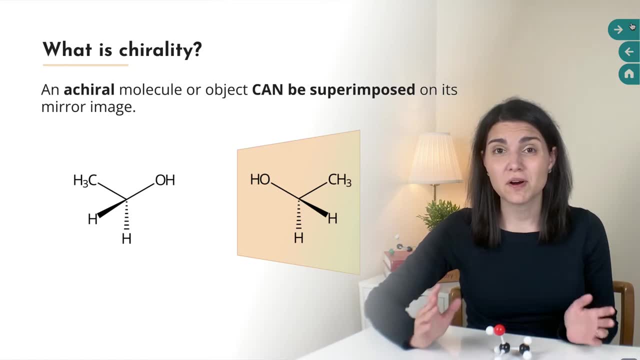 mirror images. We call them enantiomers of one another. Now, many, many molecules, especially biological molecules, have this property of being chiral, but there are also many, many more molecules that are not chiral. And if a molecule is not chiral, we call it. 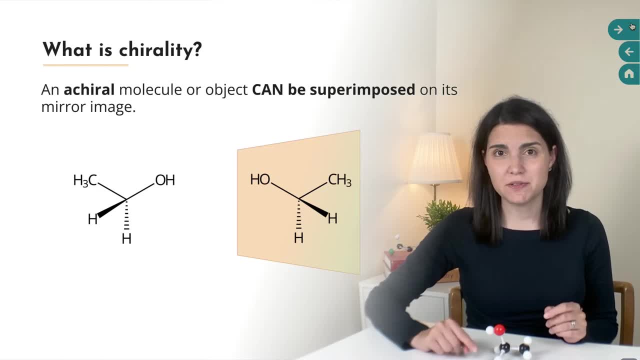 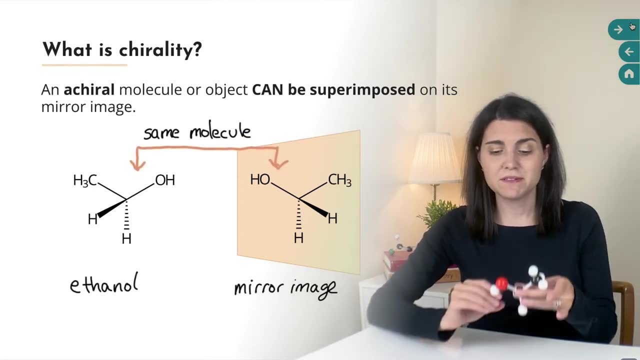 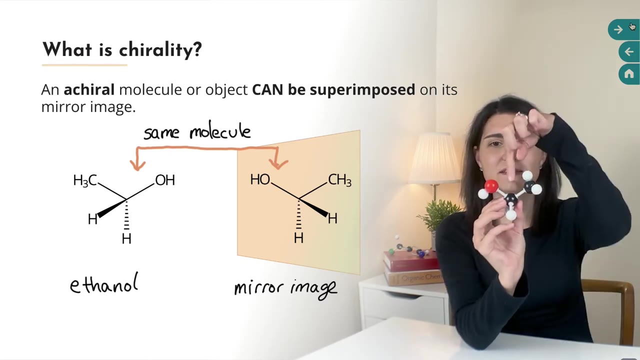 achiral. An achiral molecule can be superimposed on its mirror image. So here's an example. This is ethanol and the mirror image of ethanol. So here's a model of the ethanol molecule And if I rotate it back and forth about an axis that kind of goes through that center carbon right. 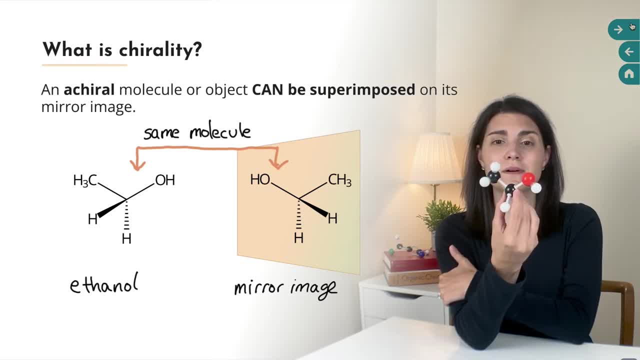 here I am generating ethanol and the mirror image as I rotate it back and forth. So that means ethanol and its mirror image are the exact same molecule, And so ethanol is therefore achiral, A skill that you're going to need in order to be able to 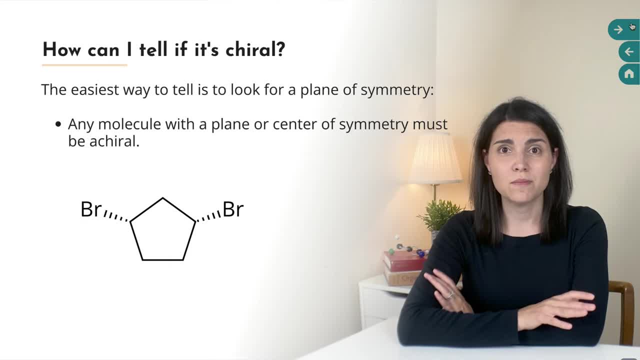 pass. organic chemistry is to be able to tell right away whether a molecule is chiral or achiral, And the quickest way to do this is to check whether the molecule has an internal plane or center of symmetry. Here's an example of an achiral molecule. 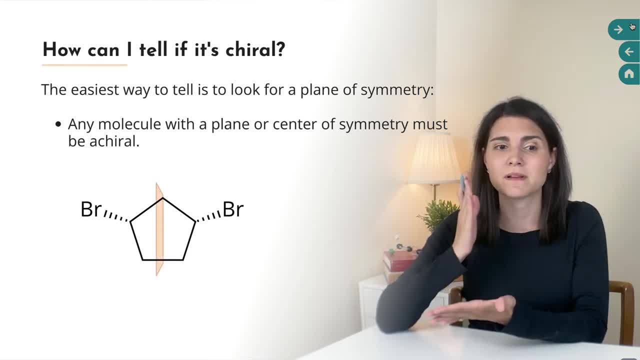 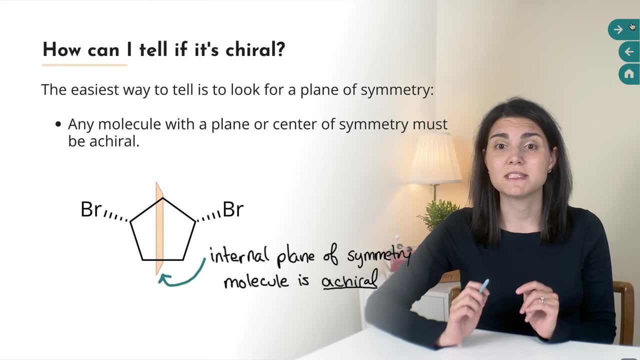 and we can imagine cutting this molecule in half through this plane in the middle And on either side you have an identical half of the molecule. So this is called an internal plane of symmetry. And because we can do this, because this molecule has that internal 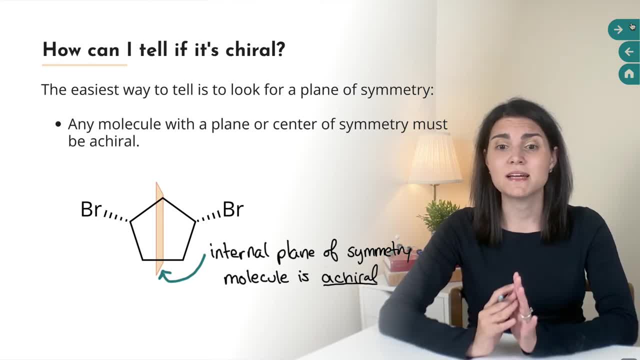 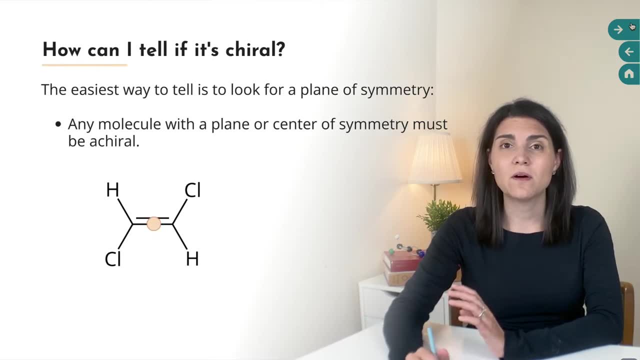 plane of symmetry, we can say with 100% certainty that it is achiral. Here's another achiral molecule. This one has what's called a center of symmetry. You might also see this called an inversion center. The easiest way to understand a center of symmetry is to think of the center. 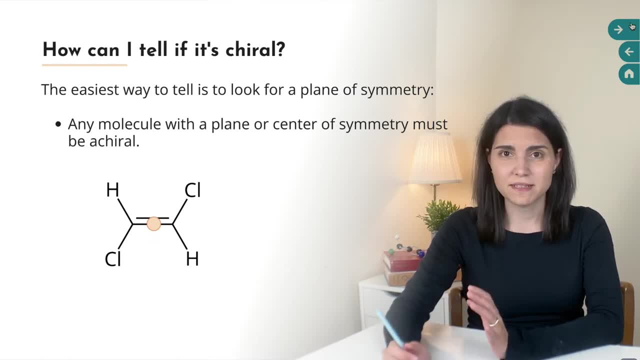 of symmetry as the zero, zero point on a coordinate system that's right in the very smack dab middle of the molecule. If you take any point on the molecule and change the sign of the coordinate, so invert them. you're going to find the exact same thing at the new point. 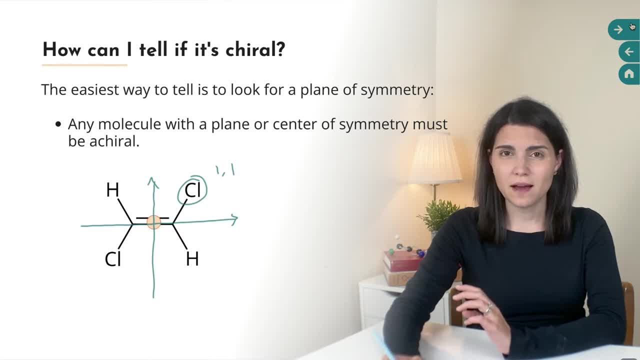 So, for example, if we say that this chlorine atom is at position one one, then we invert those coordinates to get negative one, negative one. we will also find a chlorine atom at that point, And that's true for any other point on the molecule. It can be basically reflected, right. 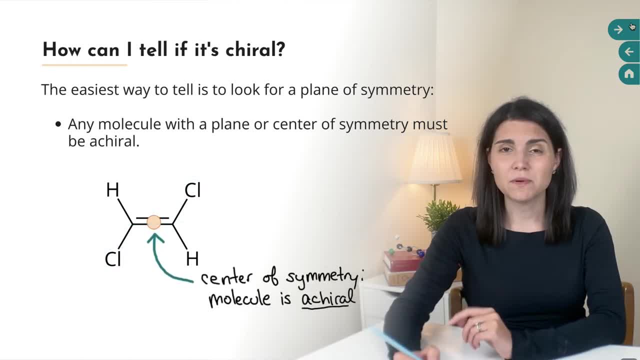 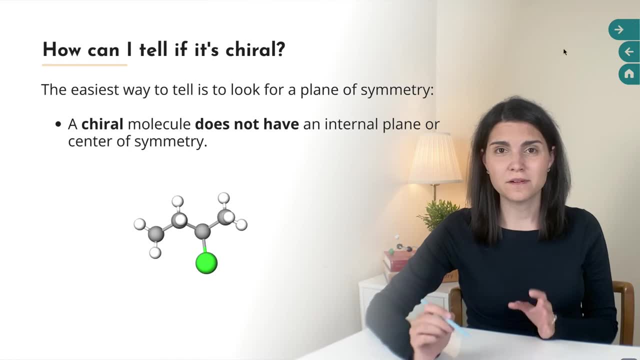 through that inversion center. Any time a molecule has a center of symmetry like that, it can be reflected right through that inversion center. Any time a molecule has a center of symmetry like this, it will be achiral. Let's bring back this 3D model of our original. 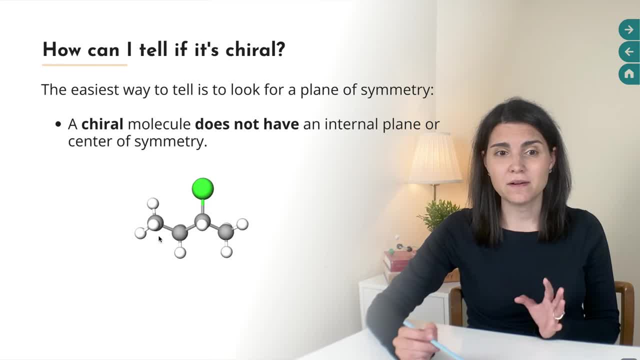 molecule 2-chlorobutane. No matter what we do to this molecule, no matter how we look at it and rotate it around and change the view, there's no way that we can find an internal plane or center of symmetry for this molecule. Any time that you find a molecule where you cannot do either of, 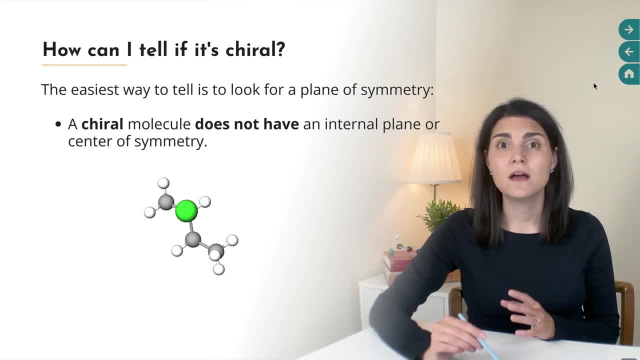 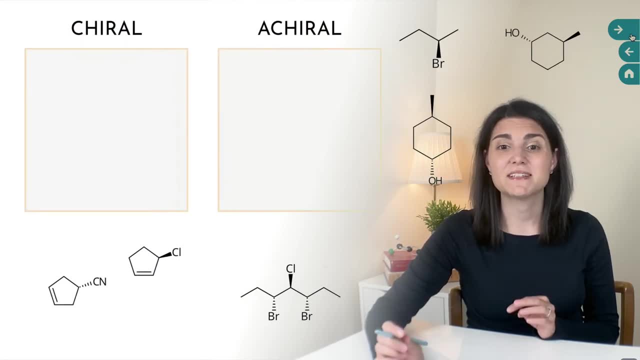 these two symmetry operations, the internal plane or the center of symmetry, the molecule is by nature a chiral, So here's a practice problem. There is a group of molecules on this slide and you need to decide whether each of them is chiral or achiral. If you're using my slides. 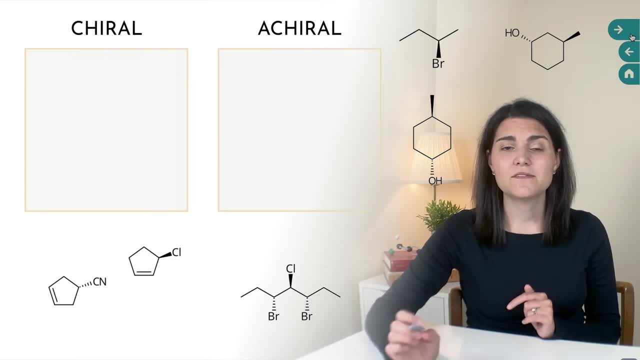 you can just pick them up and sort them into the boxes, And if you've got your own piece of paper, you can just redraw them and label them as chiral or achiral, And remember. the easiest thing that you can do is to evaluate whether each molecule has a plane or center of 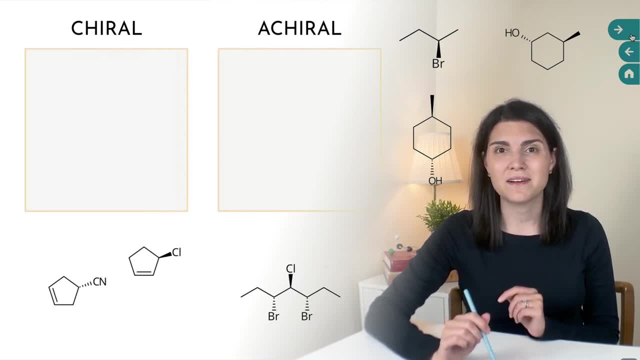 symmetry. You can pause the video now to give this a try, and I'll give the solution in just a minute. This first problem is called a chiral. This first problem is called a chiral. This first problem is trompe l'oeil. The first molecule is a chiral. It has a plane of symmetry that cuts right through. 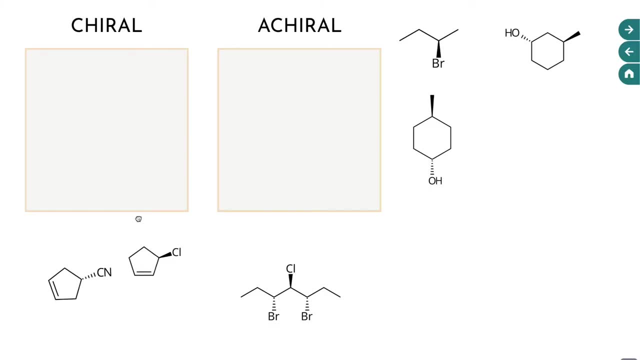 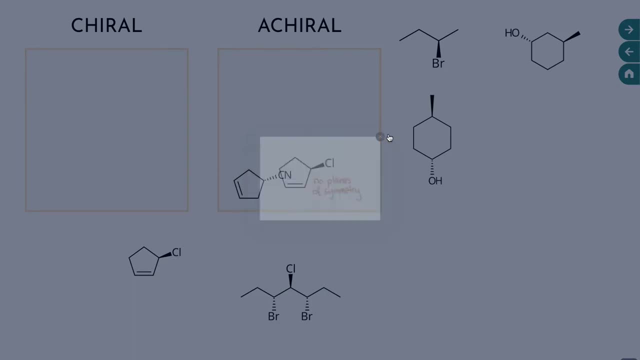 the center of the molecule through that double bond and through the CN group. This second molecule is chiral. There is no way that we can cut this molecule into equal halves and there's no center of symmetry, so this must be chiral. 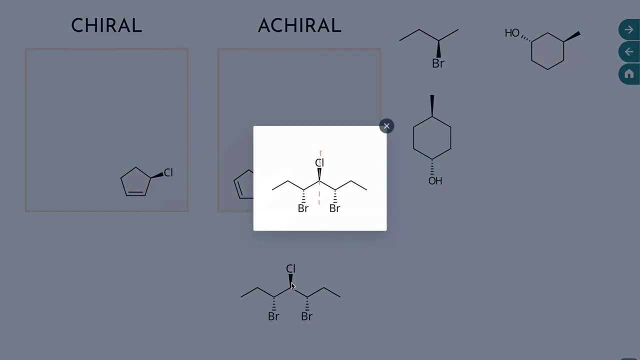 This next one has a plane of symmetry going right through the middle. That's pretty easy to see. And the next one- this sixth and seventh one membered ring- also has a plane of symmetry going right through the middle. Finally, these last two: 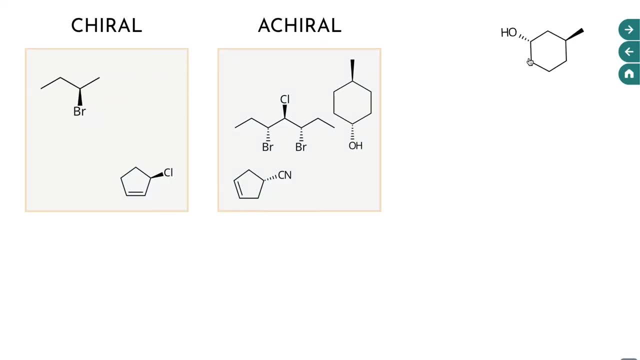 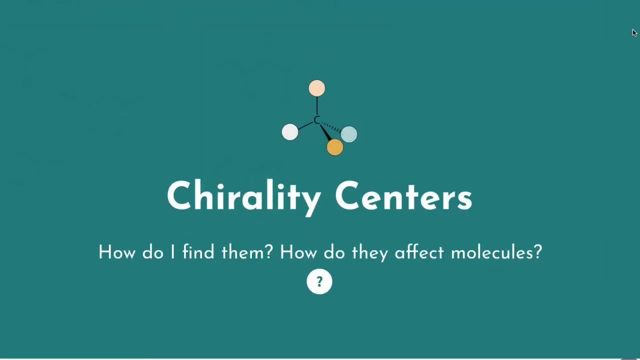 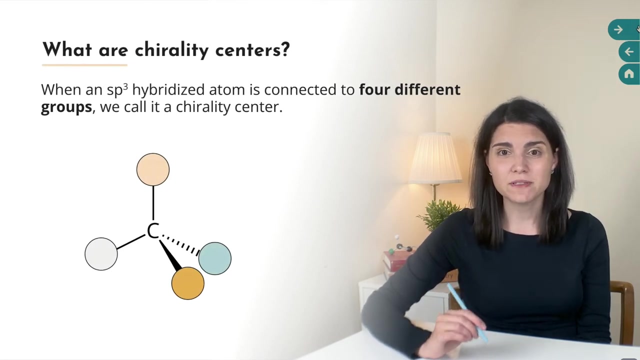 up at the top are both chiral. There's no planes or centers of symmetry on either of these molecules. Now we're going to talk about the concept of chirality centers. When an sp3 hybridized atom is connected to four different groups, we call that atom a. 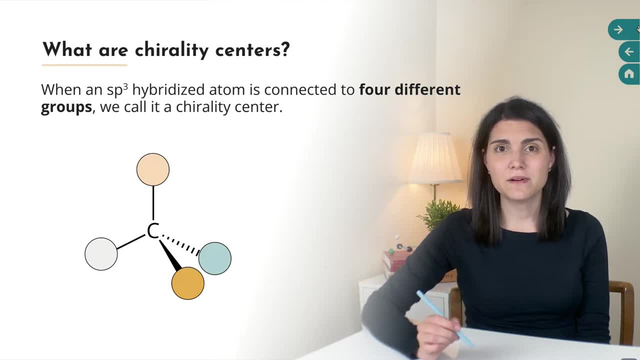 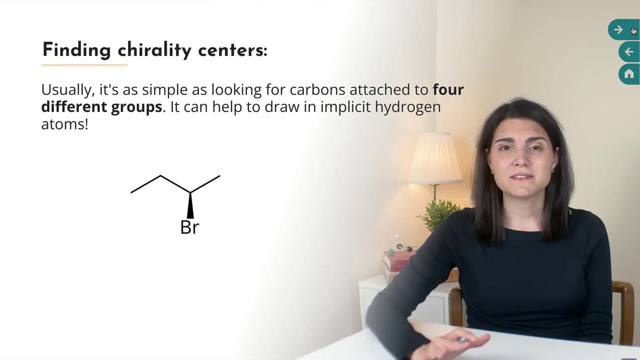 chirality center. So here we have an sp3 hybridized tetrahedral carbon atom, and it's connected to one, two, three, four different groups, and so we would say that that carbon atom is a chirality center. Usually it's pretty easy to find chirality centers on molecules. 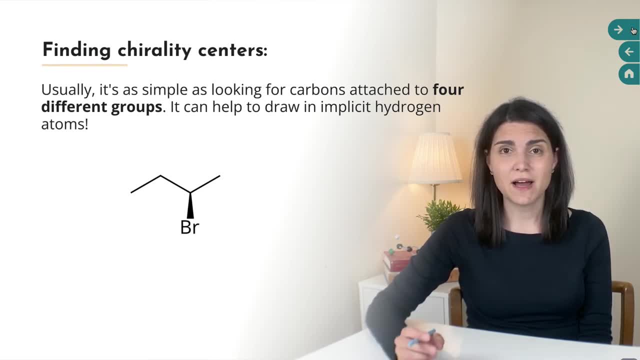 It's as simple as looking for tetrahedral atoms that are connected to four different groups. However, you might want to make sure that you remember about implicit hydrogen atoms. You can find them in the description below, If you're interested in learning more about chirality centers. 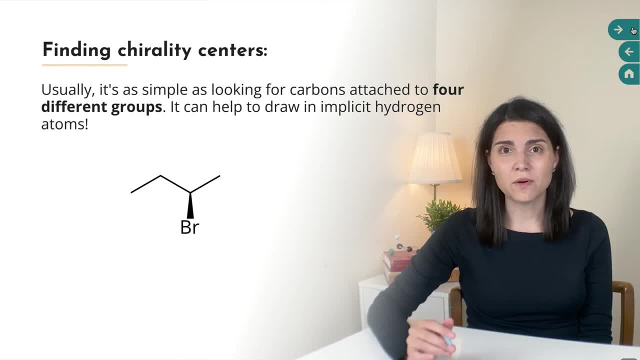 you can draw those in, because hydrogen atoms are often one of the four groups on a chirality center, but they're not always drawn in explicitly. So, for example, here's a molecule with a bromine. it's on a wedged bond, so that's bromine is pointing out at us and it's also understood that there's a hydrogen. 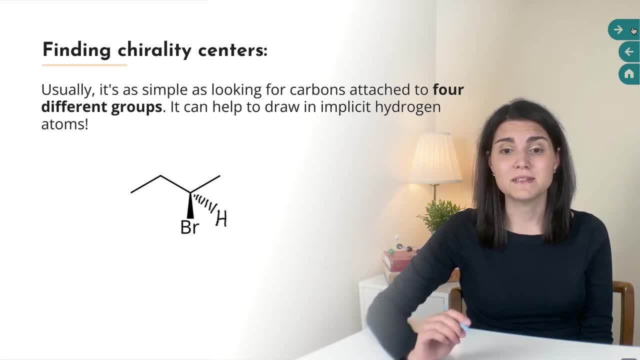 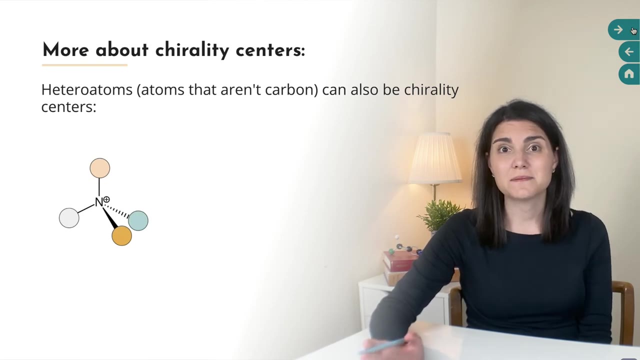 atom on that carbon as well. it would be pointing away from us into the page. So we draw it on the dashed bond, and now we can clearly see that this carbon atom is bonded to four different groups: one, two, three, four. so it is in fact a chirality center, Heteroatoms, which just means atoms that aren't 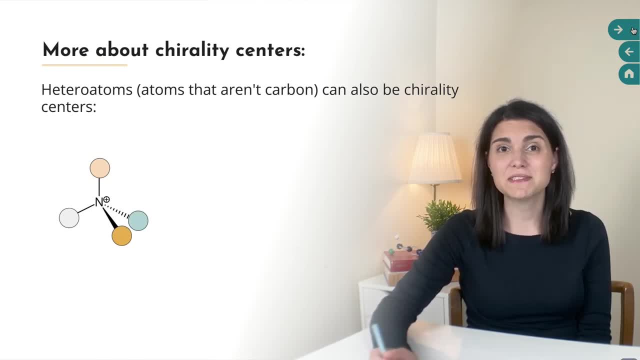 carbon can also be chirality centers. For example, positively charged nitrogen atoms connected to four different groups are chirality centers. However, neutral nitrogens connected to three different groups and having one lone pair are not considered chiral, Even though technically we can think of the lone pair as one of four different things. on that, nitrogen atom amines like 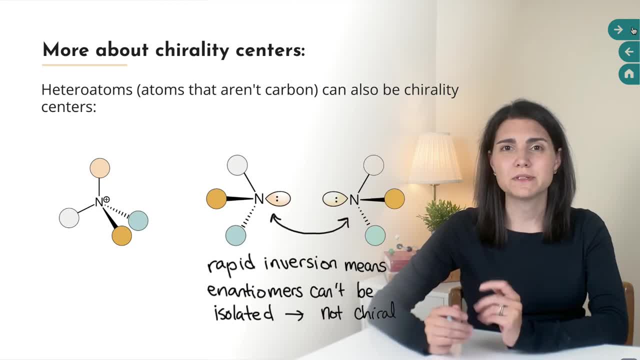 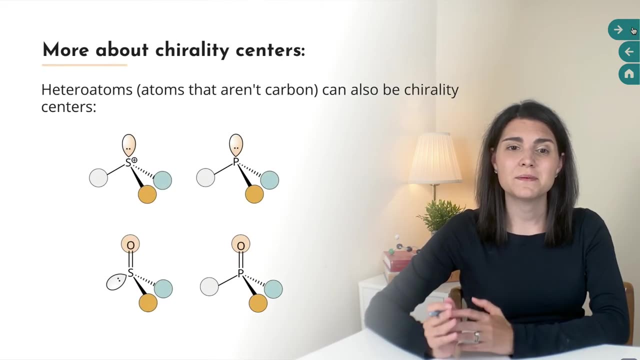 this are actually rapidly inverting at room temperature, which means that they're going back and forth between the two mirror image configurations, and so it's impossible to isolate one enantiomer or the other, so they just aren't considered chiral molecules. Here are some other examples of heteroatoms that can be chirality centers, but it's less. 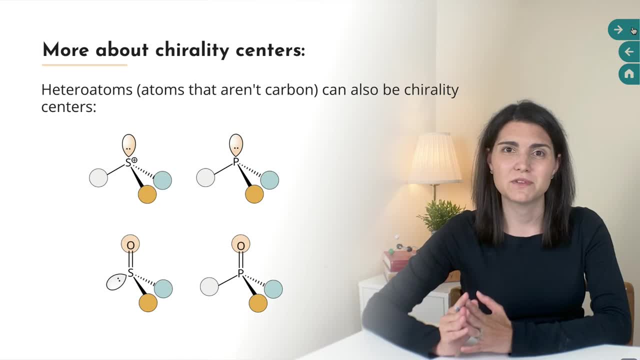 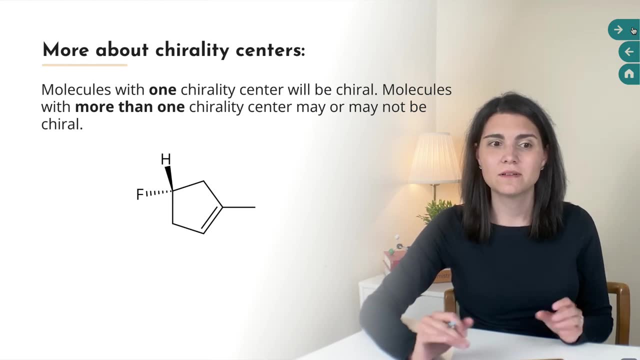 likely that you're going to run into these in your introductory organic chemistry course. It's important to clarify the difference between a molecule having chirality centers and being chiral. If a molecule has only one chirality center, it will be chiral. For example, this: 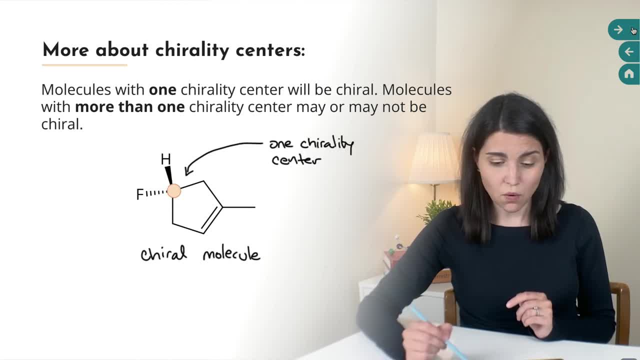 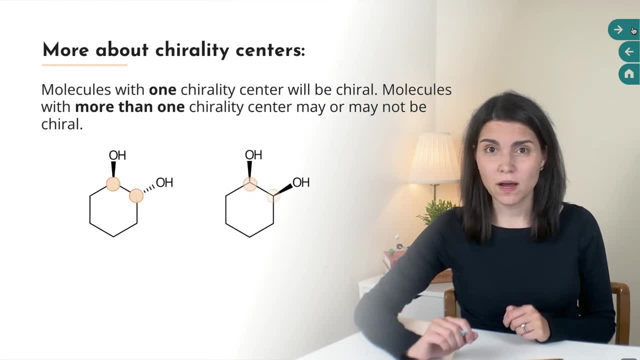 molecule below has a chirality center here and that's the only chirality center that it has. so this molecule will be chiral. However, if a molecule has more than one chirality center, it may or may not be chiral, because the way that the chirality centers are arranged could give 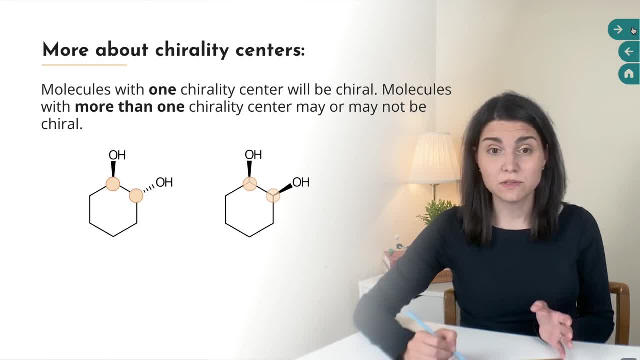 the molecule, a plane of symmetry, For example, these two molecules both have chirality centers. The molecule on the left is chiral. it has no plane or center of symmetry, but the one on the right has a plane of symmetry, so it's achiral. These molecules have a special relationship to each. 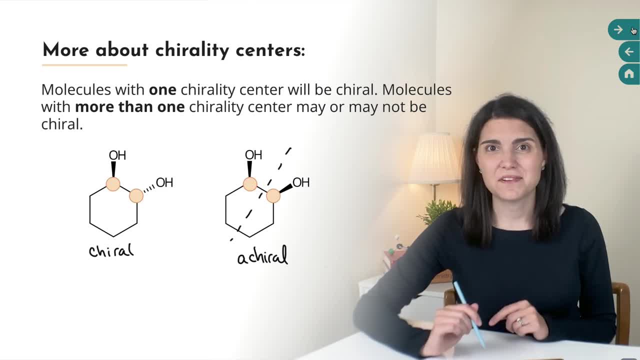 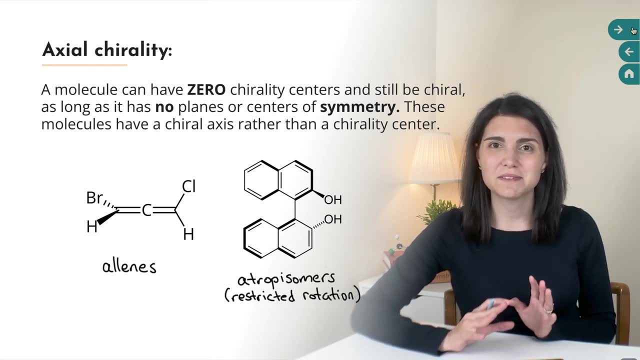 other. they're called diastereomers, and I'm going to talk about that in another lesson. Fascinatingly, it's also possible for a molecule to have zero chirality centers and still be chiral as long as it passes the test of having no plane or center of symmetry. 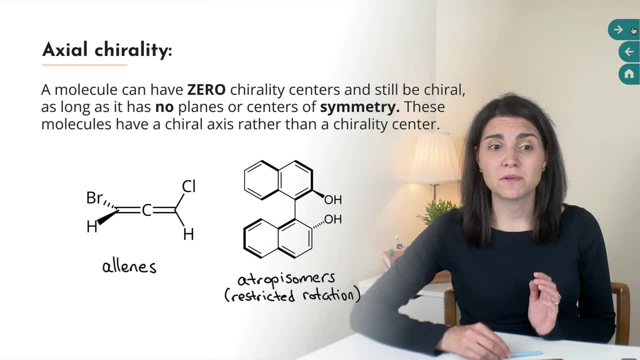 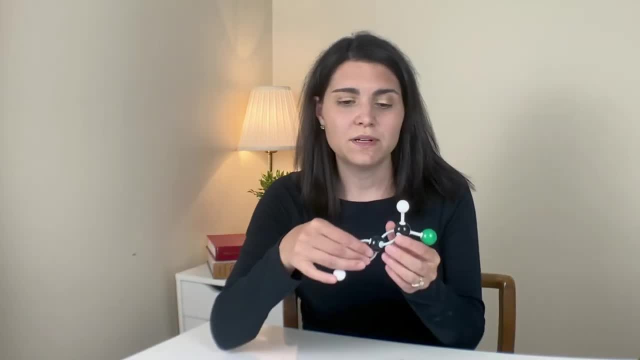 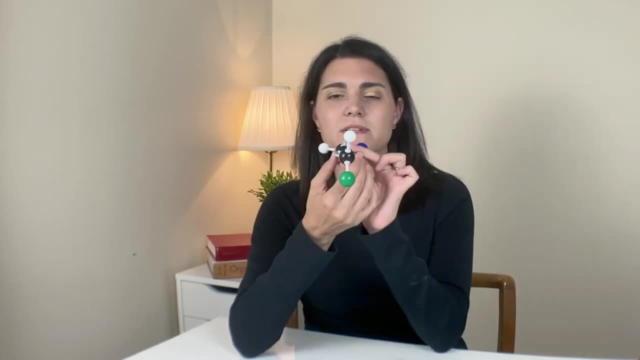 So an example of this phenomenon includes a type of molecule called an allene, where there are two consecutive double bonds. So I built an allene, and this, of course, only goes for allenes that are that have two different groups on each side of the allene, and so, as you can see, when I rotate. 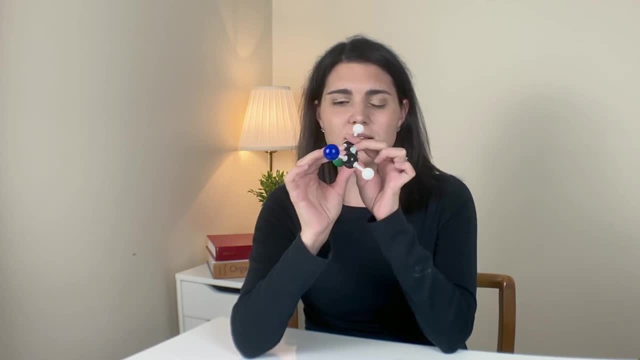 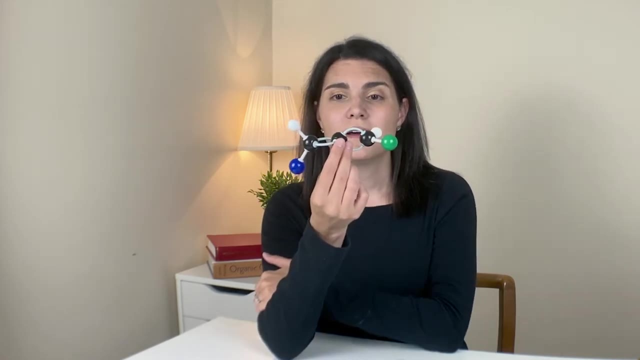 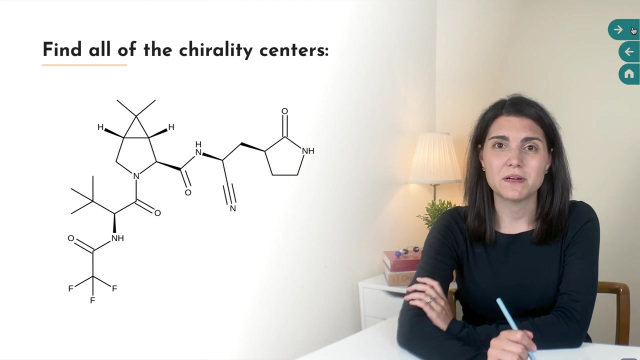 this molecule around. there's no way that we can cut this in half. There's no plane of symmetry and there's no center of symmetry in this molecule. so even though none of these carbons is a chirality center, this molecule is still chiral. Time to do another practice problem. 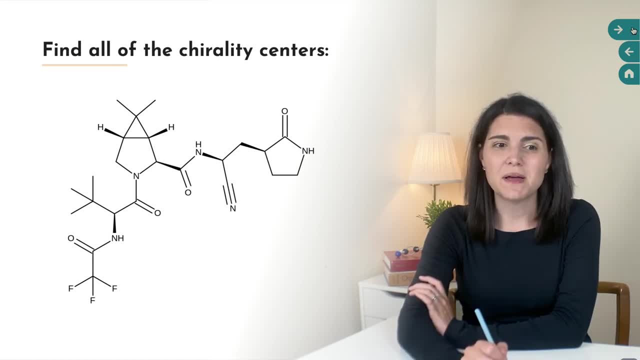 This is a giant molecule. If you know what this is, let me know in the comments, and you can pause the video now and give this a shot. see if you can identify all of the chirality centers on this great big molecule. here And here is the solution. Each of these carbons that I've circled is sp3 hybridized. 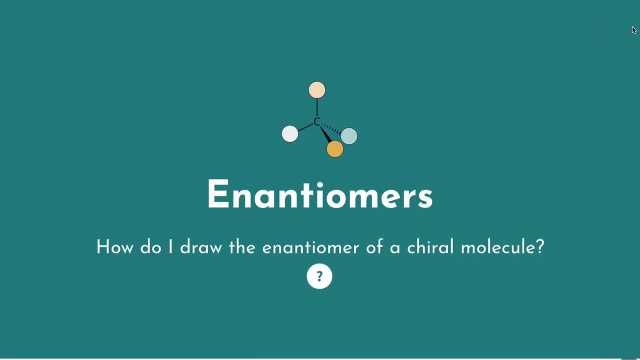 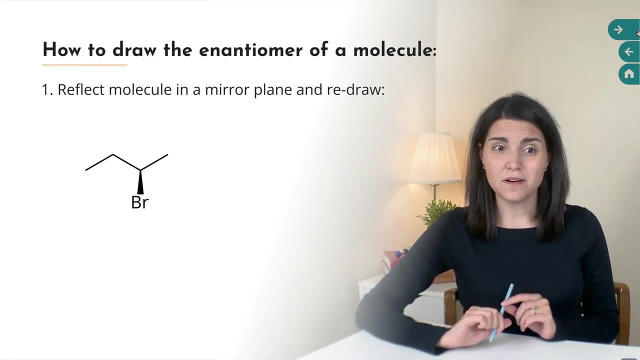 and connected to four different groups. Throughout your journey in organic chemistry, you're likely going to need to quickly draw the enantiomer of a chiral molecule, so here are two ways to do that. The first method is to reflect the molecule in an external mirror plane. So here's our chiral